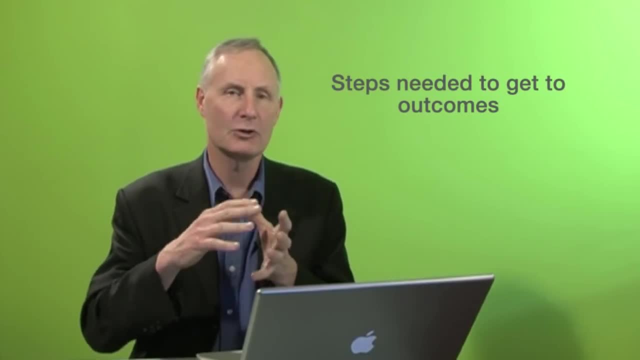 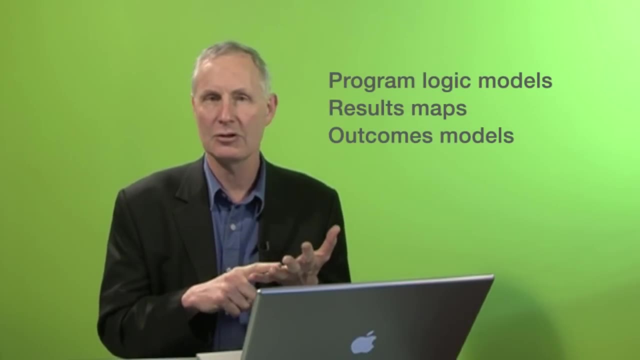 And they simply set out all of the steps which we need to take in order to get through to higher level outcomes. These things are called by a number of different names: program logics, intervention logics, results maps, outcomes models, theories of change program. 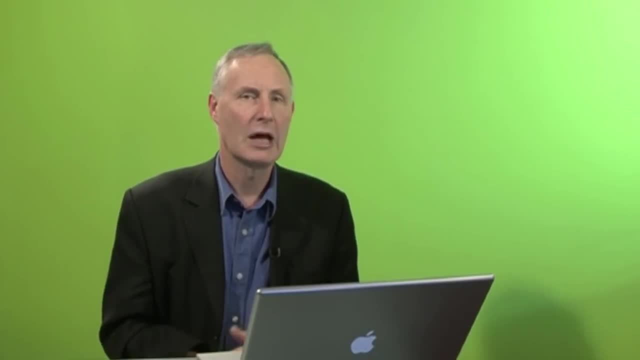 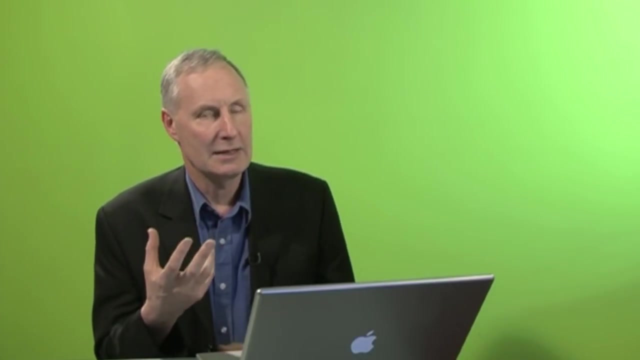 theories, strategy maps etc. But all of them have in common the fact that they're just trying to represent what is happening in a program, for stakeholders to understand that program and for program staff to work on the program. If drawn in the right way, these program logic models can be very useful for a range 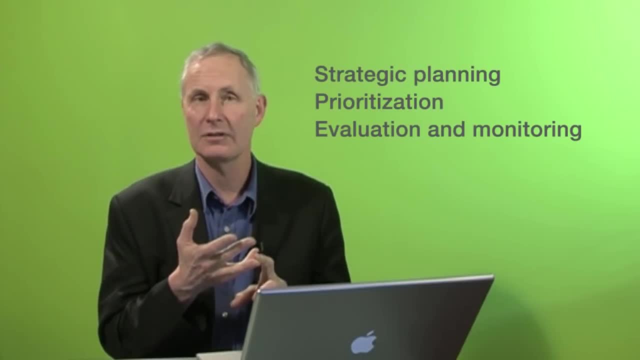 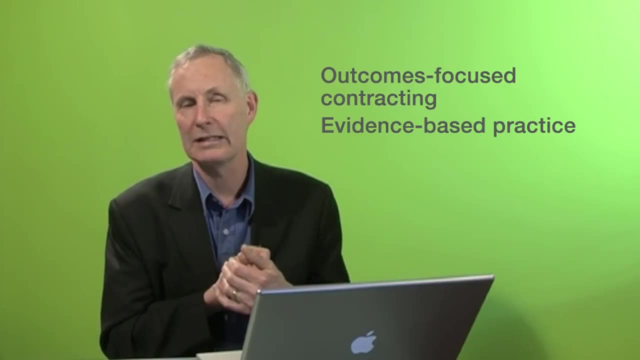 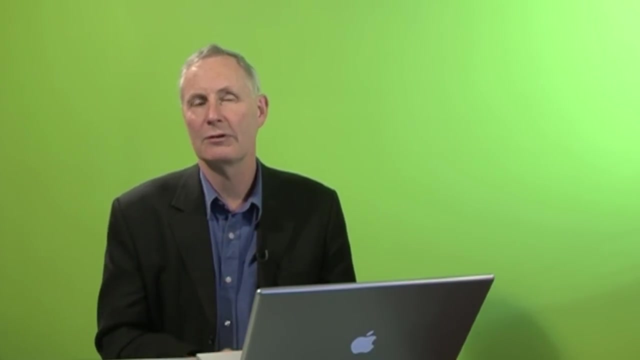 of purposes for strategic planning: prioritization, thinking about evaluation, thinking about monitoring and thinking about outcomes, focused contracting and evidence based practice. There are various ways of setting them out, and what I want to do is show you several of these ways of setting them out now, And I'm using Do You, outcomes and evaluation. 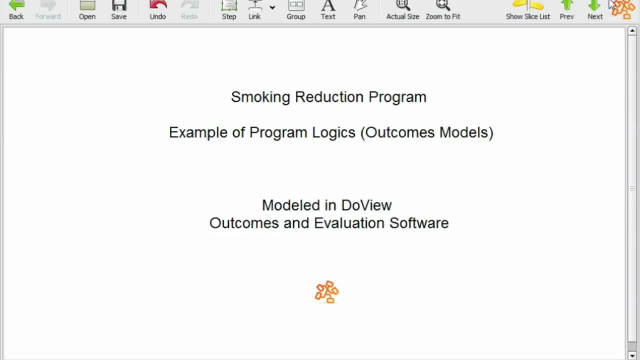 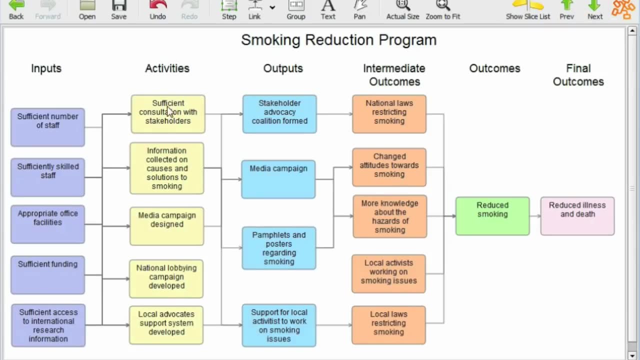 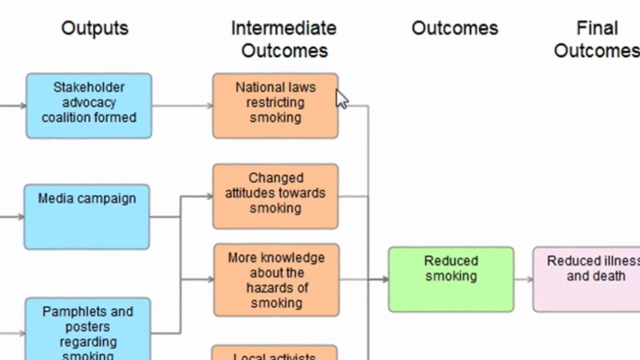 software in which I've modeled these up. One way which they're often set out is in a left to right approach, which on the left hand side, we have here the inputs and then we move through to activities, outputs, intermediate outcomes, outcomes and final outcomes in the 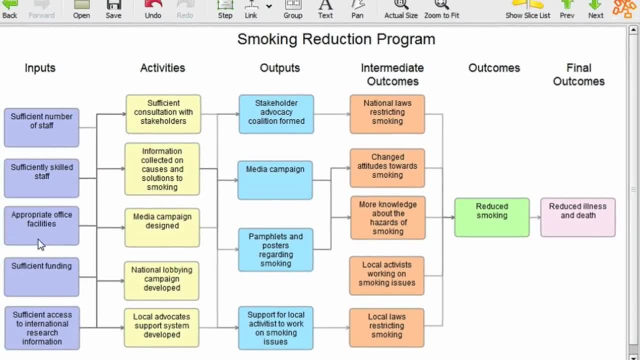 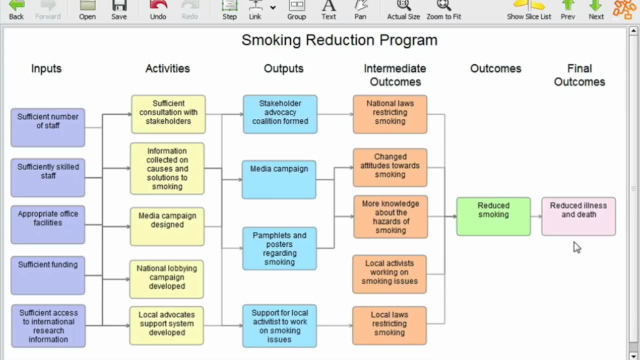 model And they start off with things that are inputs to the program, activities, etc. right through the final outcomes. In this case it's for a smoking program And the highest level outcomes are reduction in illness and death and reduce smoking and 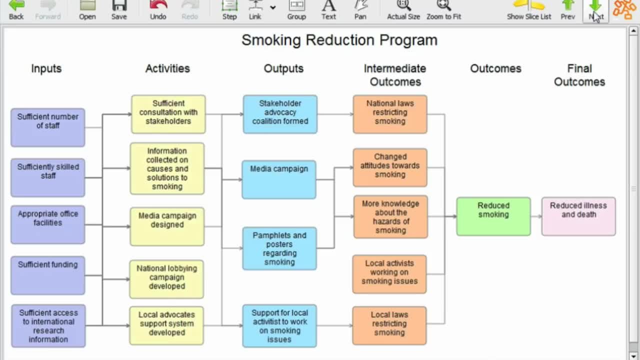 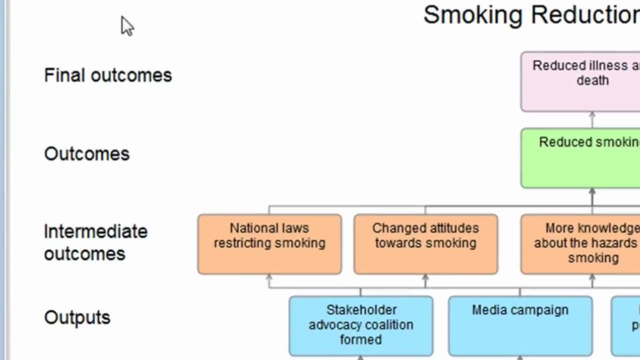 you can work back to the left hand side of the model. Another way of setting the program out is to do a top down or top up model, which sets out at the top of the model the outcomes and at the bottom of the model the inputs. 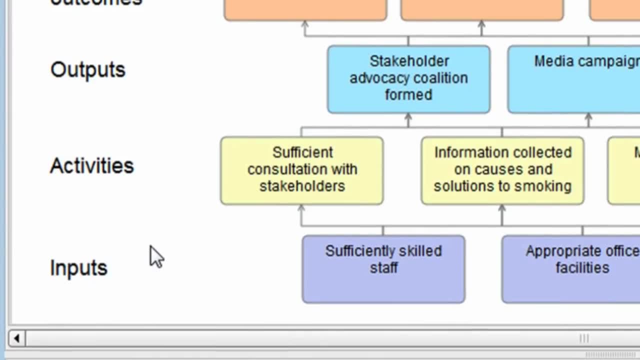 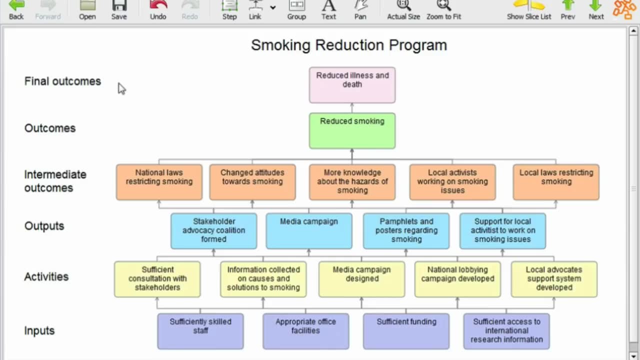 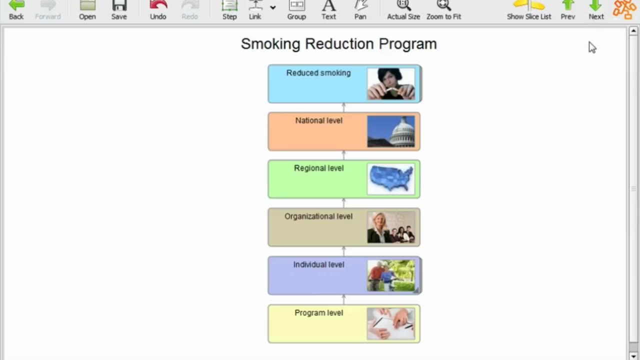 And you can see how the model which I've just showed in the left to right version here and the bottom to top version just works through the different levels of steps and outcomes which lead through to the highest levels of the model. Another way is to approach in a more free form fashion and we can see this here And 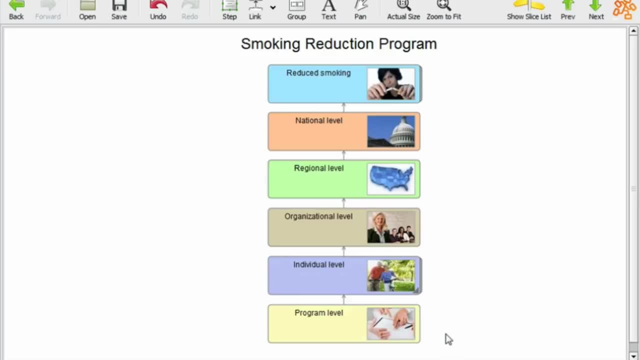 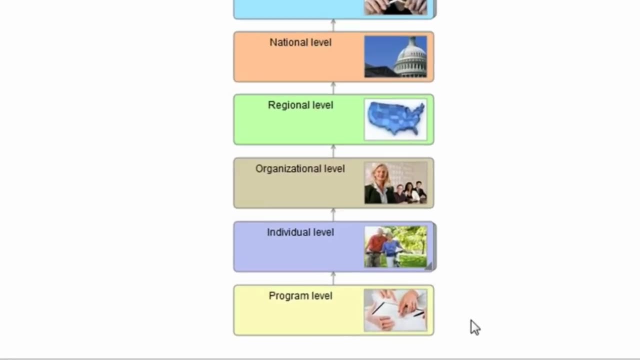 within DoView. it allows you to build modular models which can be as big as you like. So this is the advantage of not having to limit ourselves to a single page, And here we've built one which takes us through again on smoking: program level, individual level. 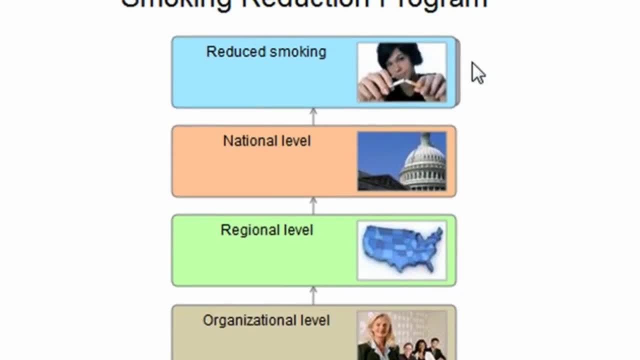 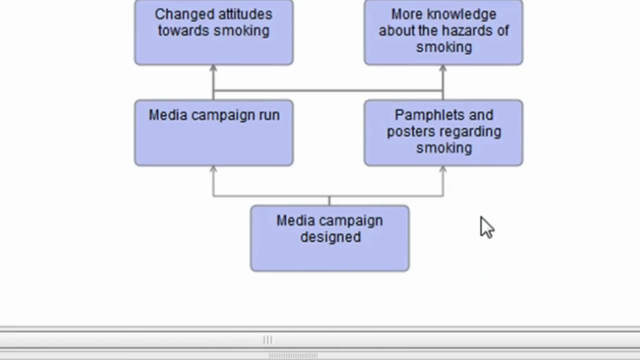 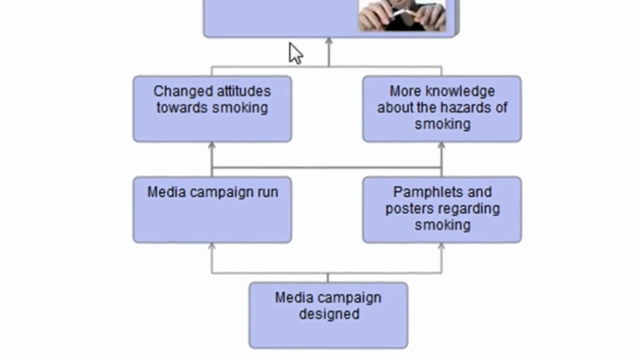 organisational level, regional, national level and up to reduce smoking. I'll just look for a moment at the individual level within the model and I've gone down to that sub page and here's a media campaign being designed being run: change attitudes towards smoking, reduce smoking. 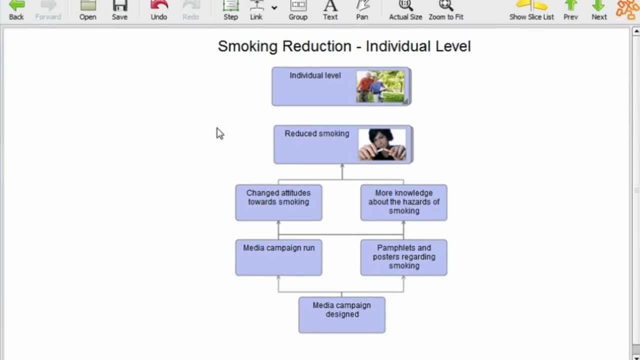 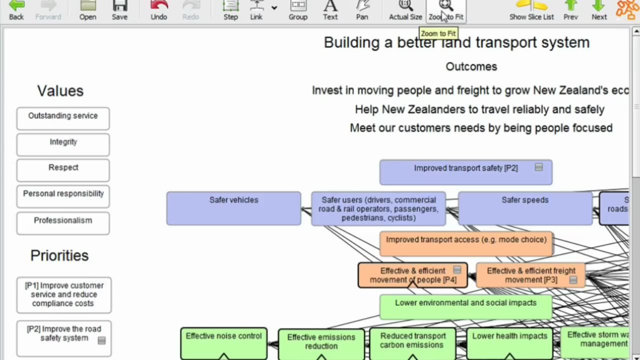 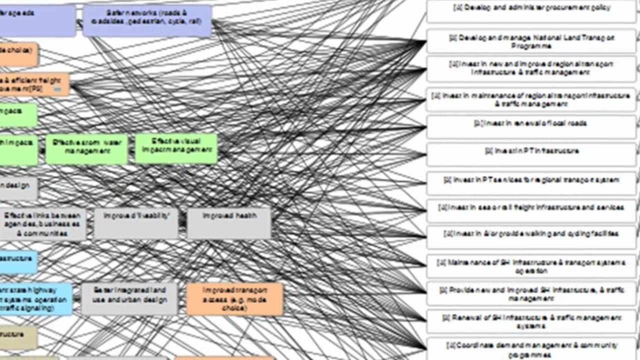 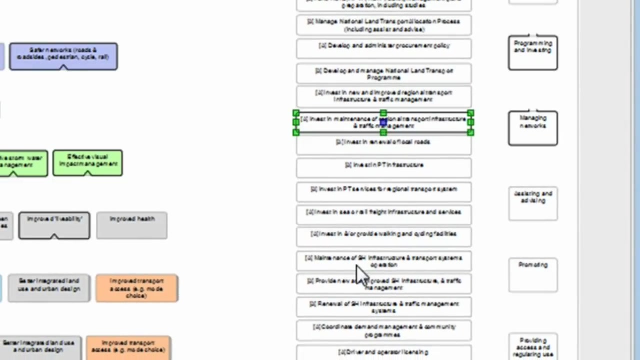 and that's the individual level of the model. We can also build big models and, for example, this one here is of a model for an entire transport system in a country and, as you can see, these models can become quite sophisticated and quite complex and it's important to be able to break them down and view 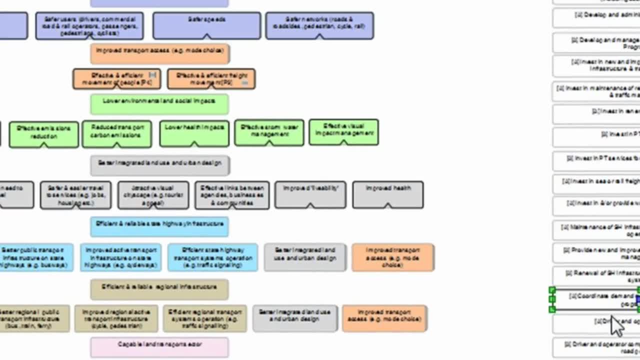 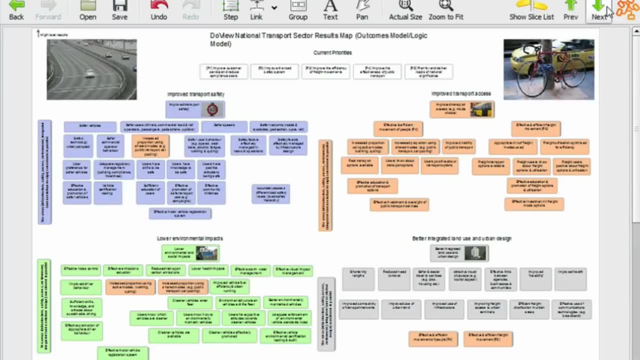 them in various ways which make them efficient to work with, and we can, if we're using something like Doovoo to do that. This last model I want to show you is a poster version of the transport system model and, as you can see, this is 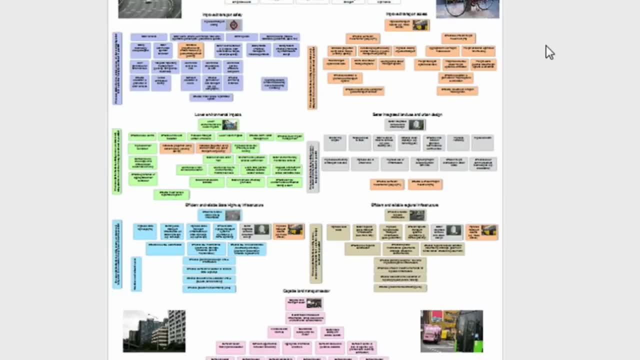 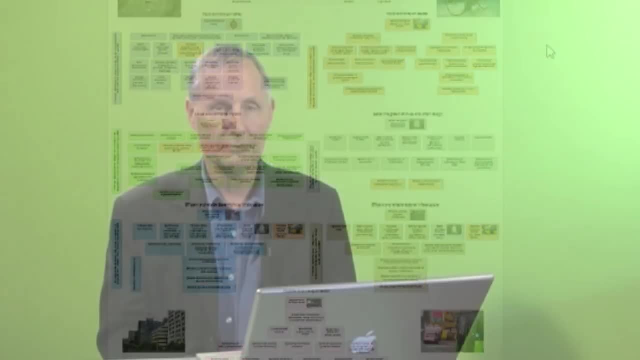 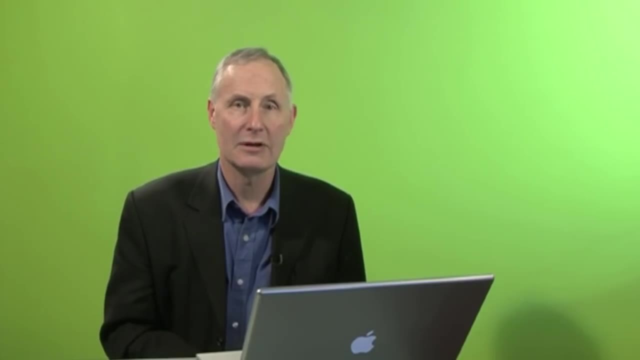 designed to print out on paper and it could be put on the wall for organisational staff to look at the outcomes which are being achieved by this particular model. So program logic models or outcomes models and results maps etc are a really useful way of communicating what it is you're trying to do, and I hope. 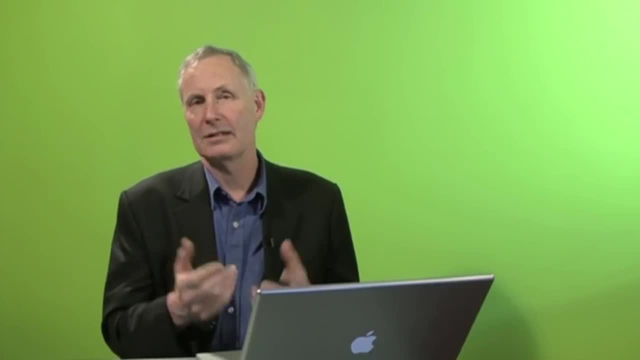 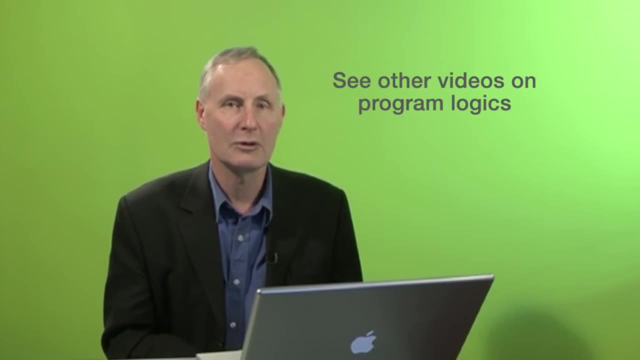 that this brief introduction will give you some insight into how they can be used. I'd suggest that you look at the other videos in this series which look in more detail at how you can work with program logic models, and I have developed a set of 13 tips which you may be interested to look at in the next. 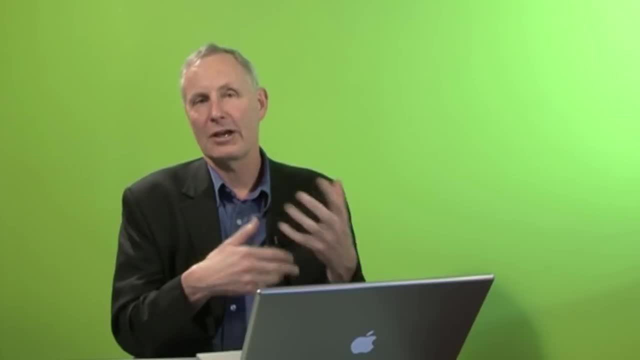 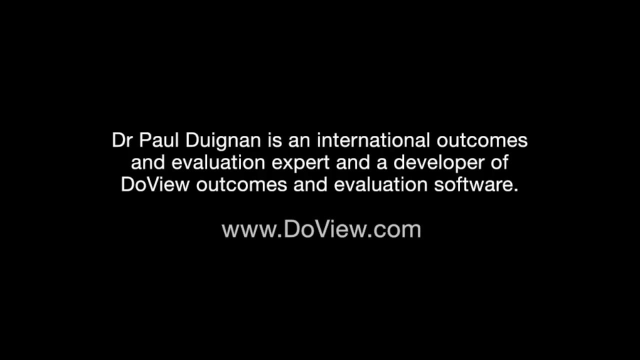 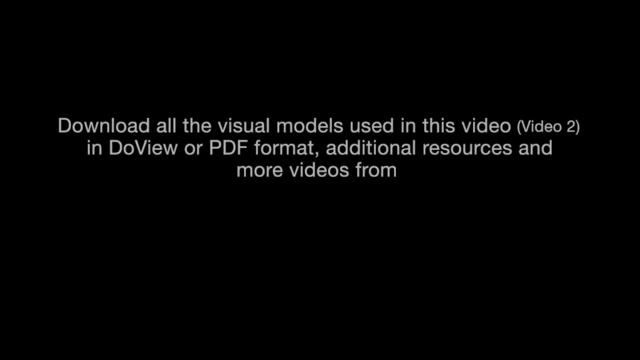 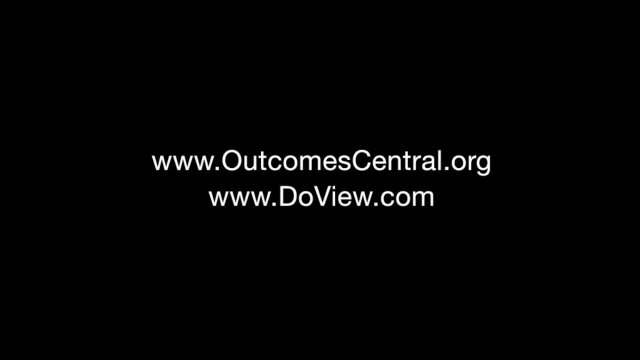 video which help you build these models in a fashion which makes them useful for a range of purposes. so if you have any questions, please feel free to reach out to me and I'll be happy to answer any questions that you may have, and I'll see you in the next. video.